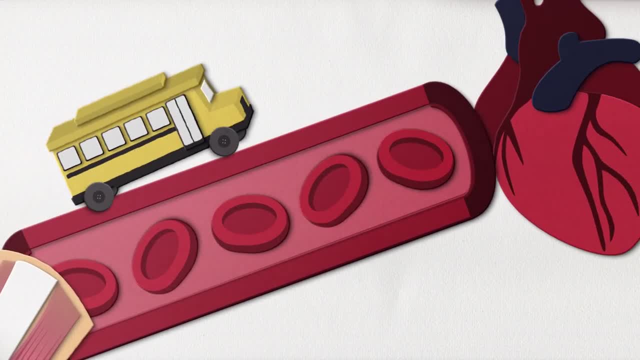 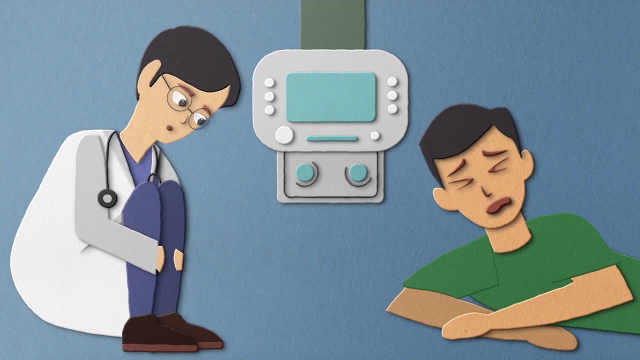 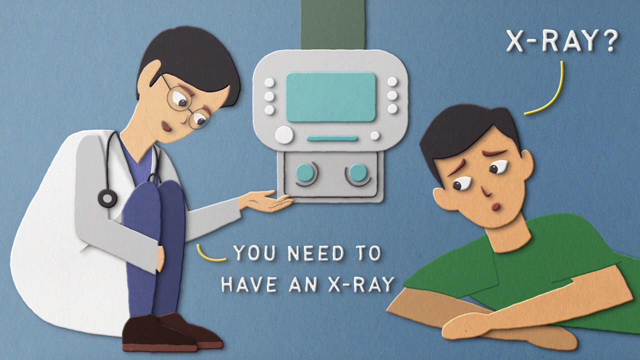 explore different bones, muscles, blood vessels and organs without having to perform surgery. Most people will be introduced to medical imaging when a doctor asks them to have a scan to investigate a source of a symptom, injury or pain. But what kinds of medical imaging techniques are? 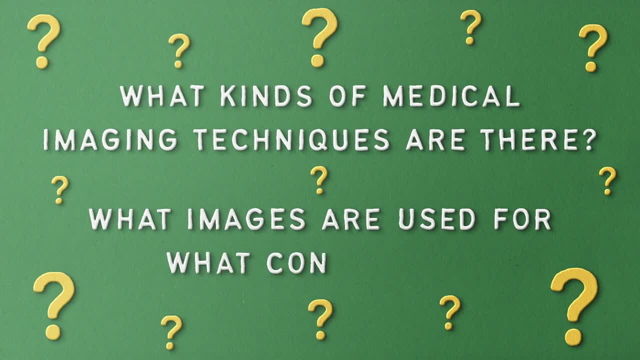 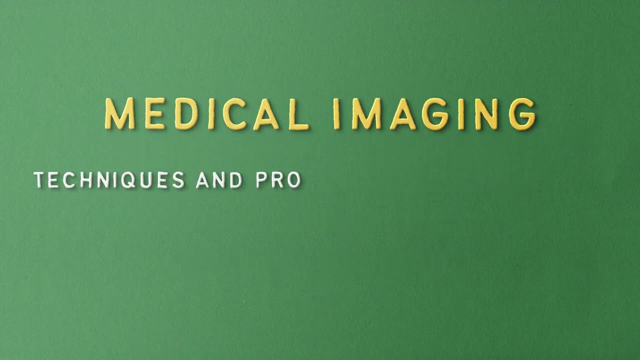 there, And what images are used for what conditions. To get these answers and more, stick around as we learn more about them. When we say medical imaging, we're referring to techniques and processes used by many different types of healthcare professionals to create images of various 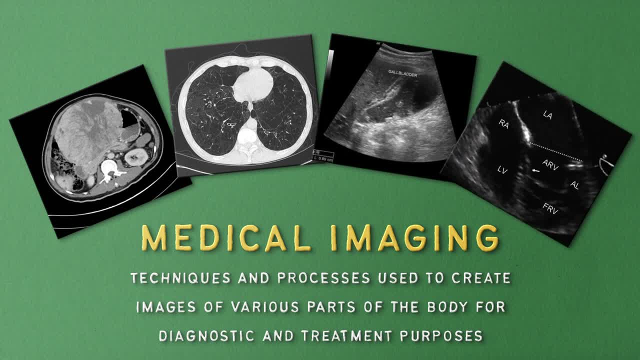 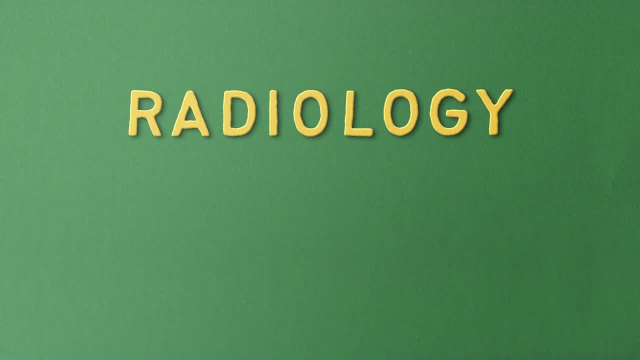 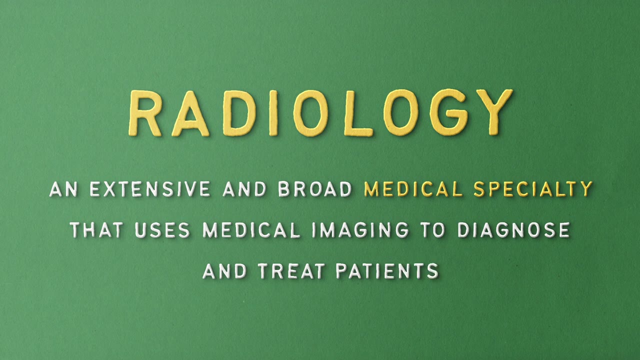 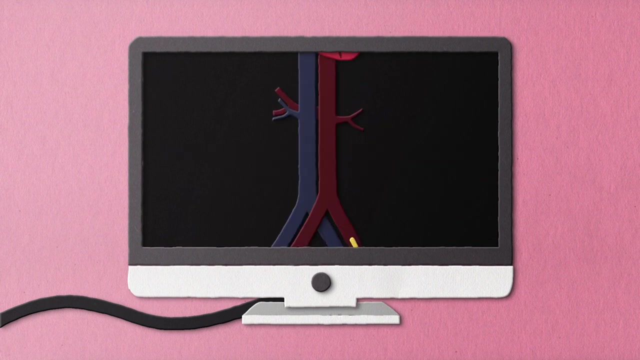 parts of the body for diagnostic and treatment purposes. Not to be confused with radiology, Radiology is an extensive and broad medical specialty that uses medical imaging to diagnose and treat patients. Medical imaging techniques are used by healthcare professionals for many reasons. These techniques may be used to help doctors find their way when introducing 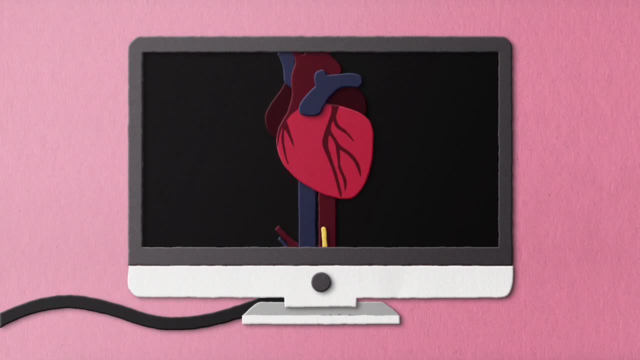 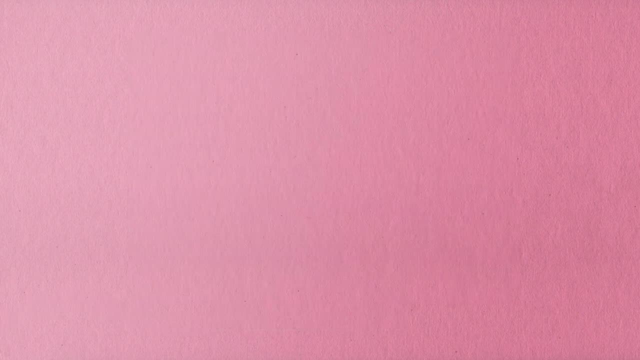 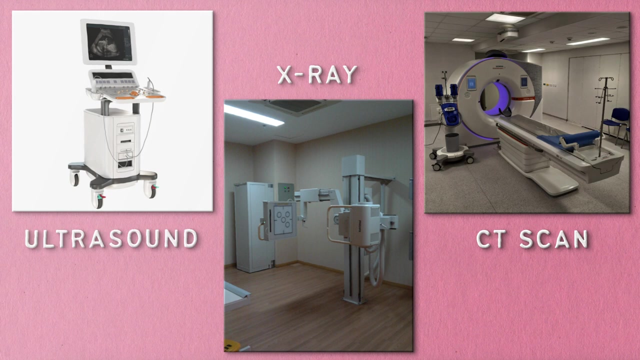 catheters or needles in your body. If medical imaging did not exist, they might end up poking something they shouldn't. Medical imaging tests like CT scans, x-rays and ultrasounds are done to screen for health conditions before symptoms appear. diagnose a potential cause for existing. 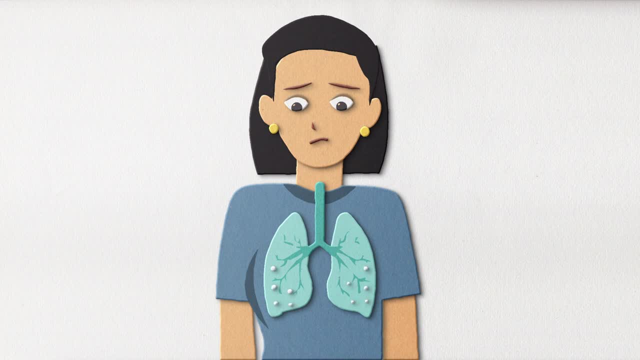 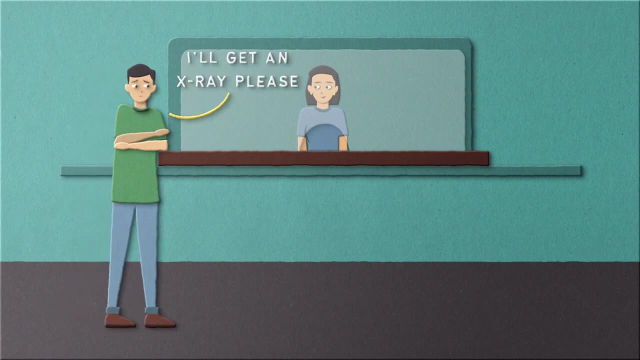 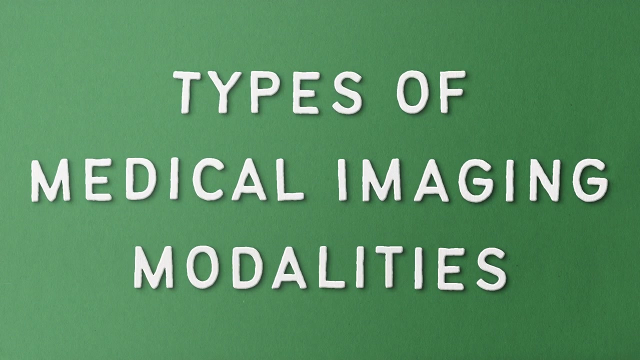 symptoms or even monitor an ongoing condition. Medical imaging test results are crucial in helping healthcare professionals decide the best treatment options for each patient. Okay, now that we know what medical imaging is and why it's so important, let's explore some of the 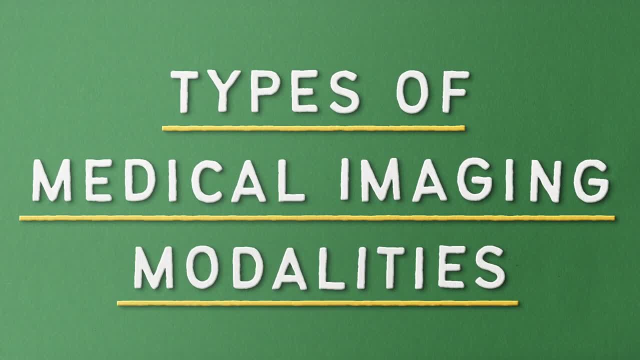 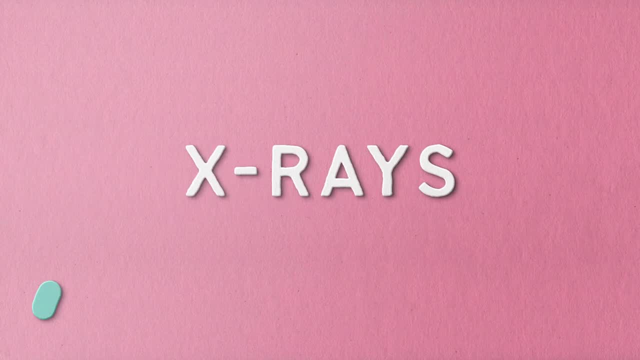 most popular types of medical imaging techniques in the world. Let's start with the most popular types of medical imaging modalities and find out why we need them. First on our list, x-rays. X-rays are a type of electromagnetic radiation just like the visible. 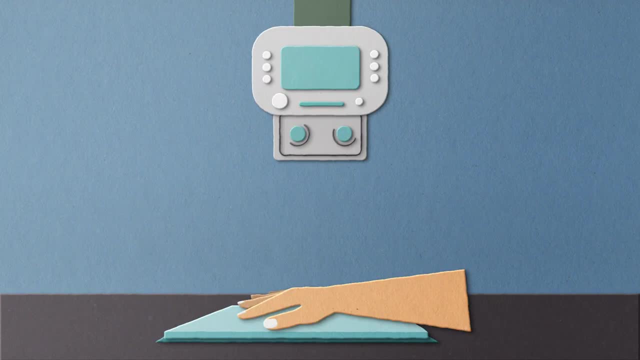 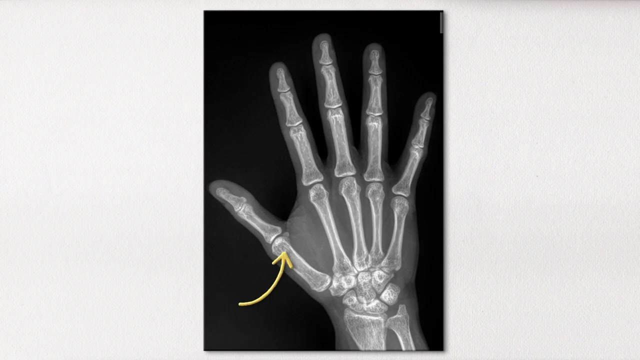 light you see all around you. The test works by firing x-rays at a part of your body and using a film called x-ray detector to capture the x-rays that pass through your tissues. The denser area of the x-ray detector is where the x-rays absorb more of the x-rays and appear lighter, white or light. 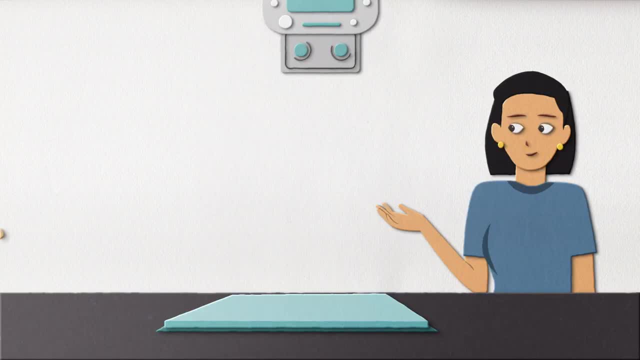 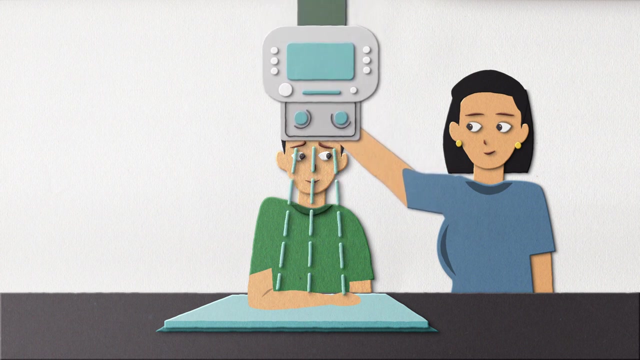 gray on the image. X-ray tests are widely available and commonly used as a diagnostic technique, particularly for orthopedic issues. So every time you have a problem with your bones or joints, you will probably have to have some x-rays shot through you. But don't worry, when done in a clinical setting, it's all safe. 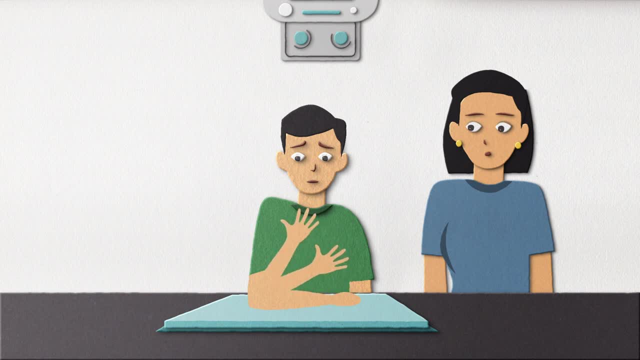 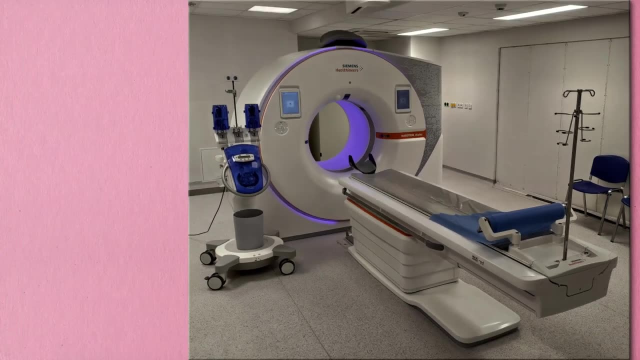 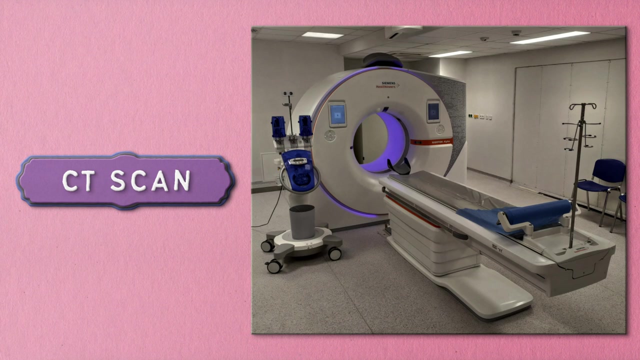 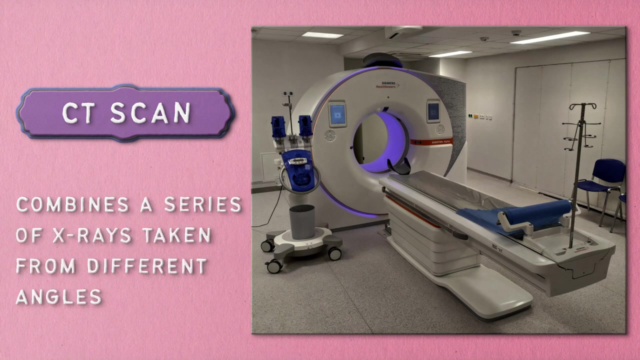 You won't grow an extra limb or acquire a superpower, even though it would be cool. Next on our list we have CT scans. A CT scan or CAT scan is short for computerized axial tomography scan, and it combines a series of x-rays taken from different angles. 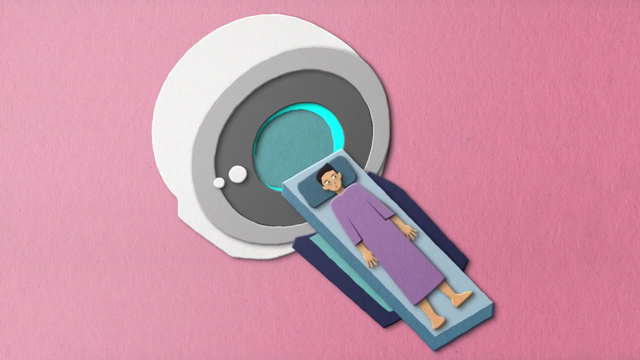 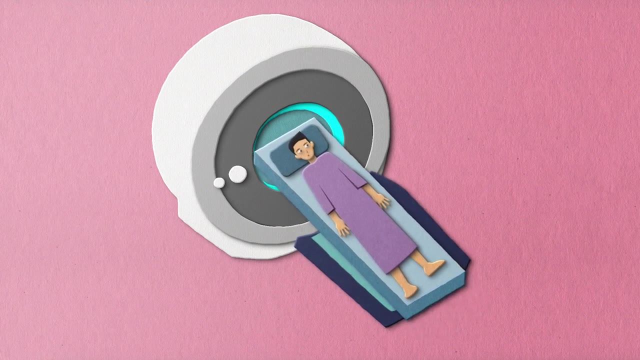 The patient is asked to lie on a narrow table that slides into the x-ray detector. The patient is asked to lie on a narrow table that slides into the x-ray detector, The CT scanner, which looks a little like a giant donut. The scanner contains rotating 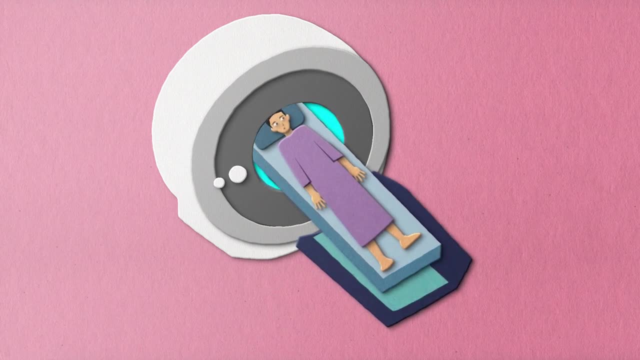 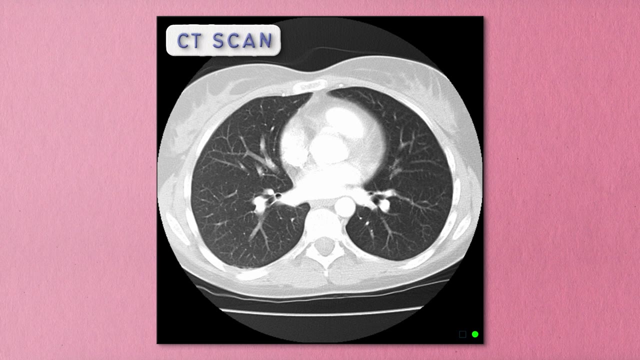 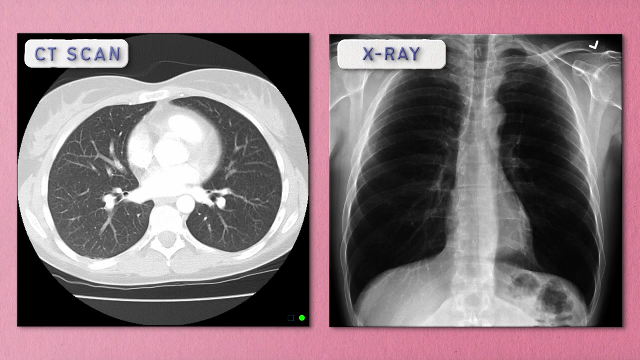 x-ray machines that produce a cross-sectional image, which results in a 360-degree view of the body. CT scans produce much more detailed images than regular x-rays and can actually take an image of internal organs. In some circumstances, the patient is also given a contrast dye, which helps. 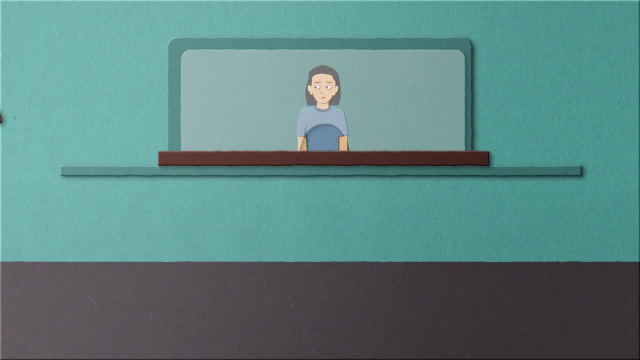 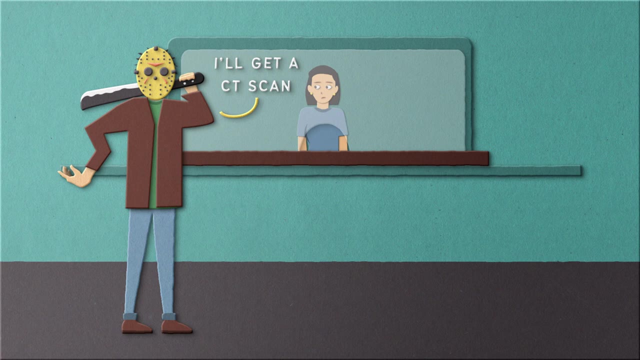 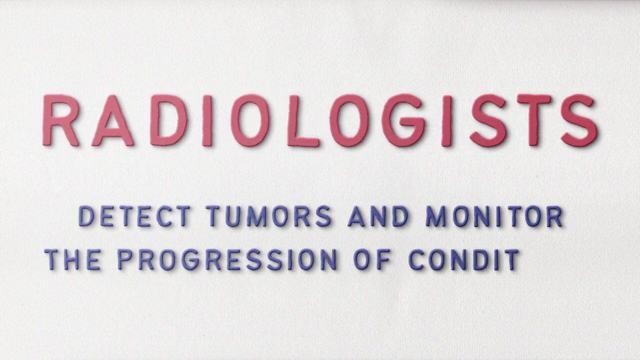 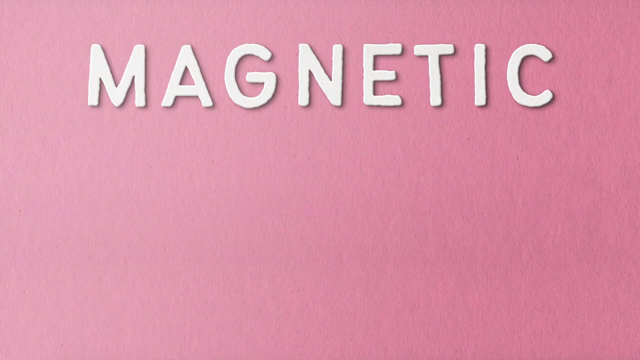 outline softer tissue CT scans are typically used for complex bone and joint problems like complicated or unusual fractures. Radiologists can also use them to detect tumors and monitor progression of conditions like heart disease, emphysema or liver growth. We're moving on to magnetic resonance imaging, also known as MRI. 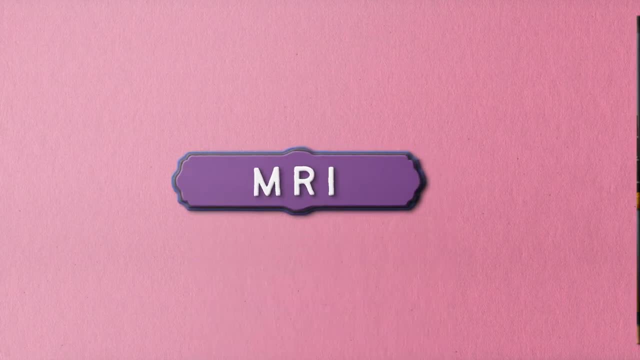 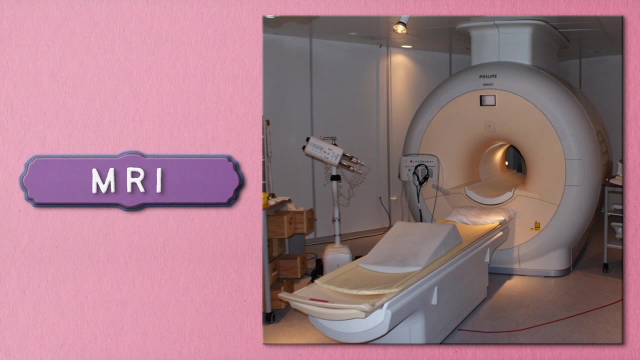 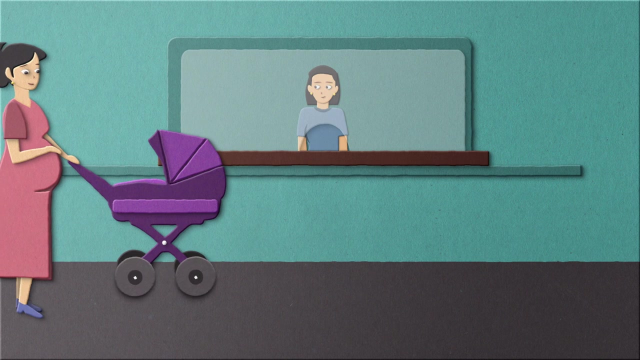 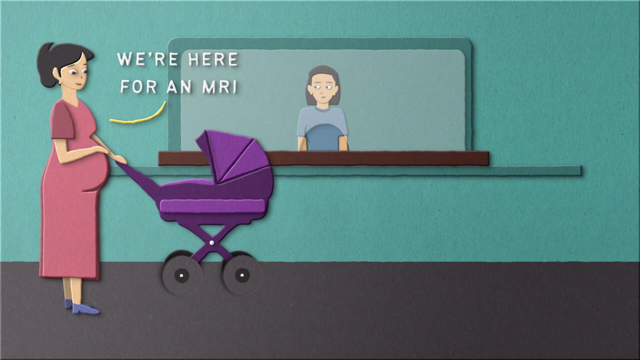 Like CT scanners, MRI scanners produce cross-sectional images of your body. They provide, however, a superior quality when it comes to image detail. Another great advantage of MRI scanners is that, unlike CT scanners, they don't rely on radiation, making them safe to use on pregnant women and babies. MRI scanners use a combination of powerful 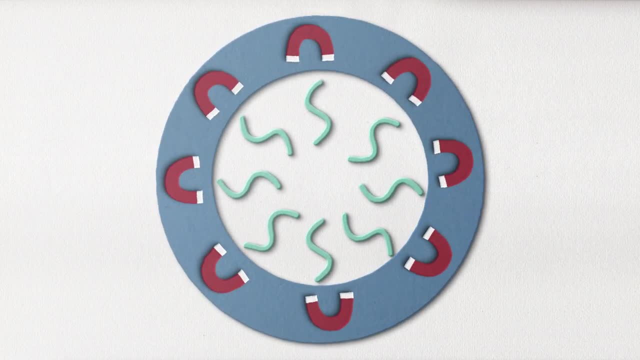 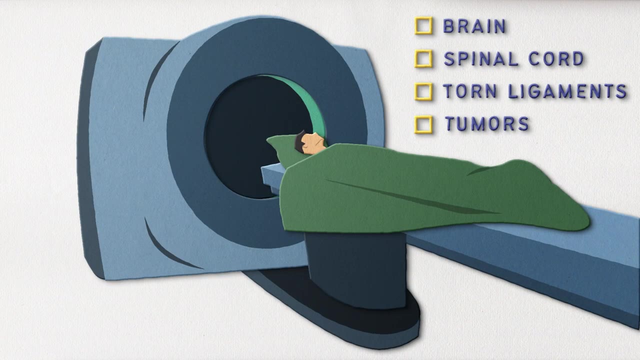 magnets and a magnetic resonance sensor. These magnets and radio frequency waves to generate an image of the body. They're especially useful for examining the brain and spinal cord, as well as torn ligaments and tumors. Another thing about MRI scans is that they are incredibly noisy- like standing next. 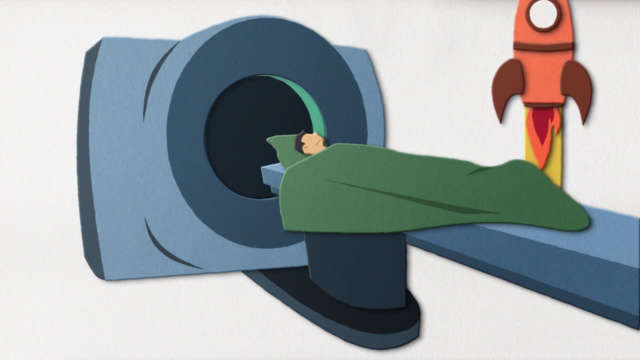 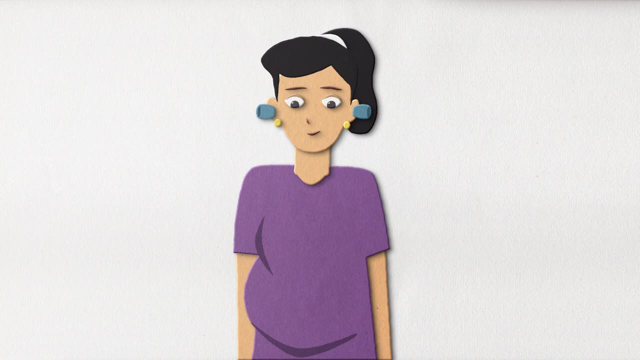 to an airplane during takeoff type of noise. For that reason patients are given earplugs. There are also other safety concerns with MRI scans Because they use powerful magnets. patients have to let the radiologist know if they have pacemakers or metal in their bodies. 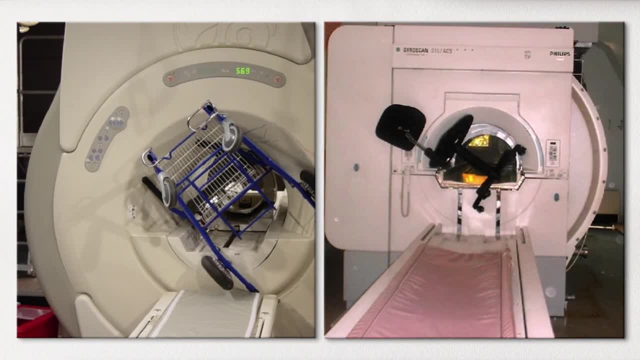 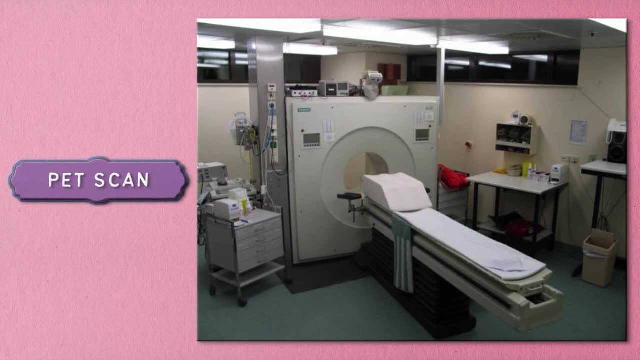 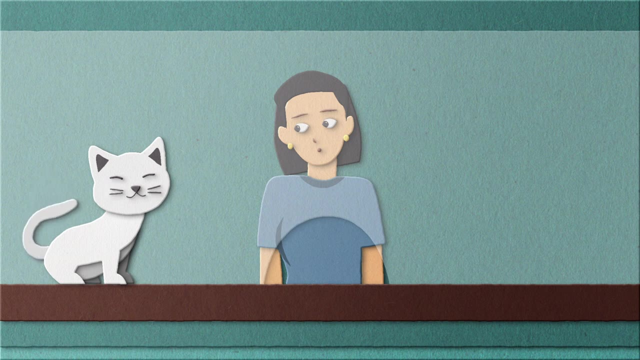 so they can avoid things like this from happening. The next medical imaging modality I want to talk about is PET. No, it does not involve using a cat or dog to diagnose something. PET stands for Positron Emission Tomography, And, even though it's not as popular as the other, 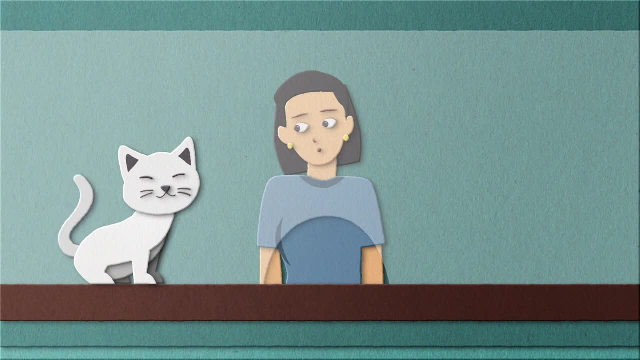 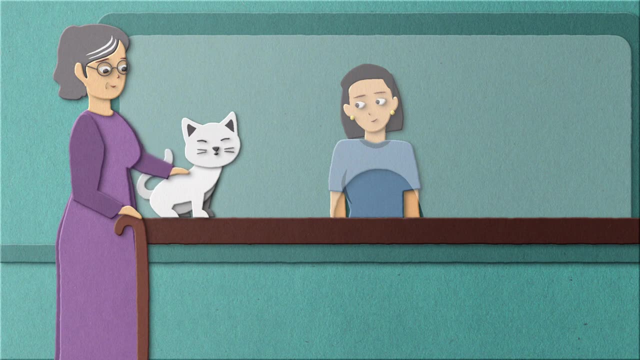 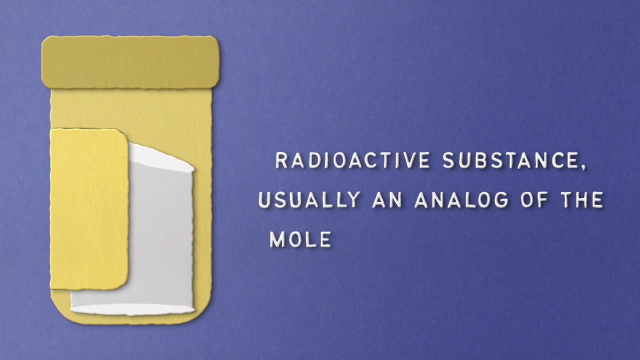 medical imaging modalities, it is still a very important one. PET scan is often used in the diagnosis and monitoring of cancer and neurologic diseases like Alzheimer's. It uses a radioactive substance, usually an analogue of the molecule glucose, called tracer, and a scanner to examine how your tibia is. 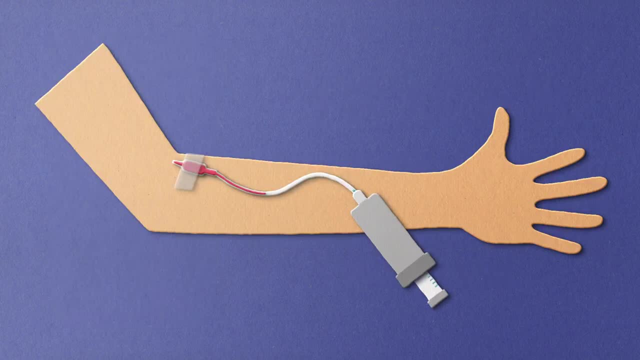 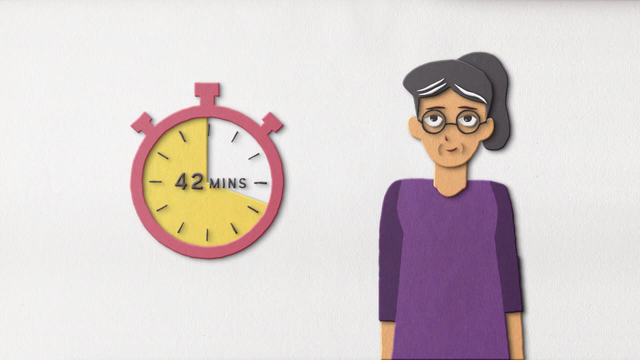 The scan is usually done in the form of an X-ray of the tissue or organs functioning. Typically, the tracer is injected into the patient's vein so it can travel around in the blood. It usually takes around one hour for the tracer to be absorbed by your body, and then the 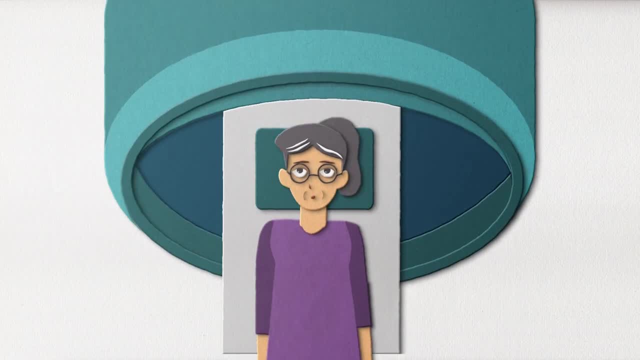 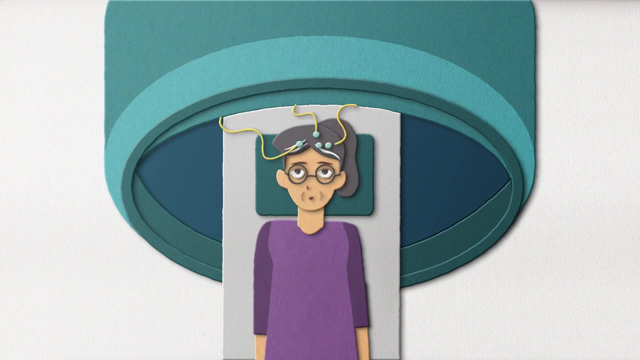 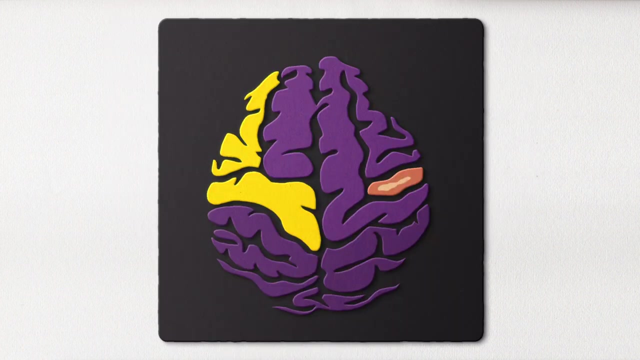 scan can begin. During the actual scan you lie on a narrow table that is inserted into a tunnel shaped scanner. The scanner detects the radioactive signals emitted by the tracer and converts the signals into a 3D image. The tracer will be absorbed by different parts of the body in 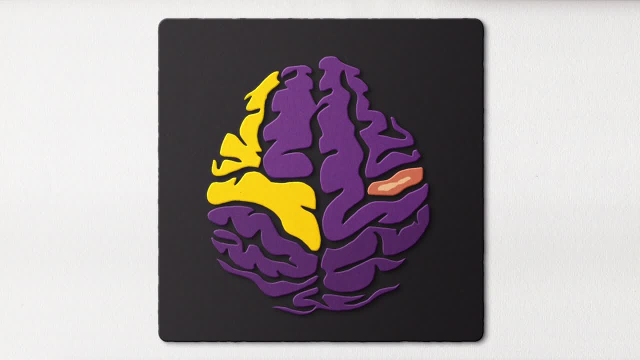 varying amounts, and that will allow doctors to see which areas show abnormal metabolic activity, which is usually the case for cancer cells. So PET scans allow healthcare professionals to find the location of a tumor or spot other areas where the cancer may have spread to. And what's great about PET scans is that they are safe for. 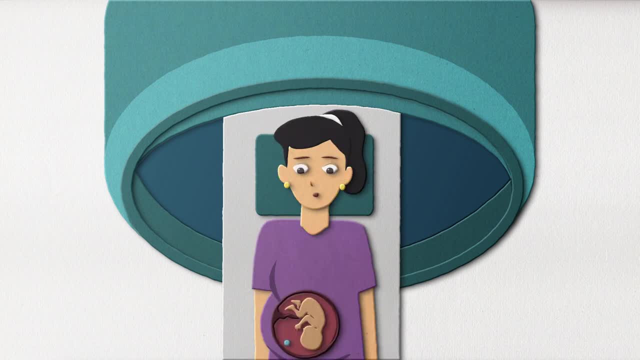 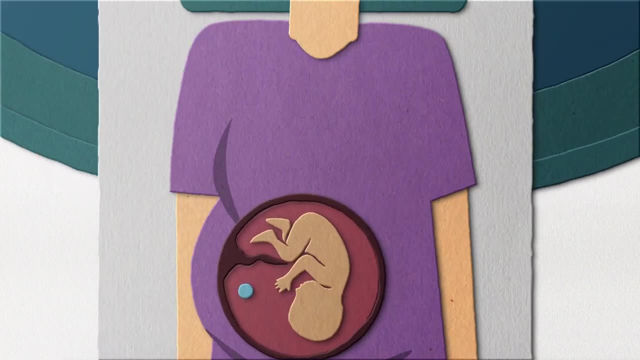 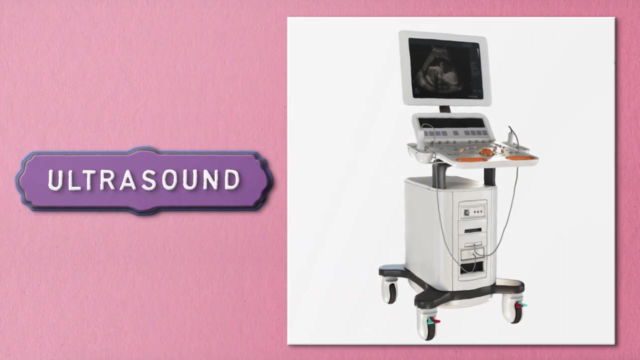 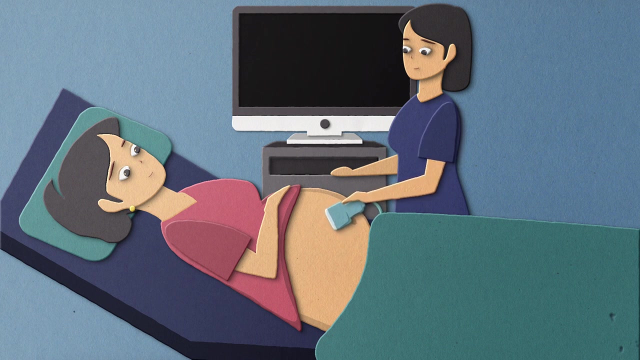 the majority of patients. The only exceptions are pregnant women or women who are breastfeeding, due to the possible risks of the radioactive tracer in the development of the baby. We couldn't talk about medical imaging without mentioning ultrasound. People usually associate ultrasound to pregnancy follow-ups, but due to their non-invasive and non-radioactive nature, 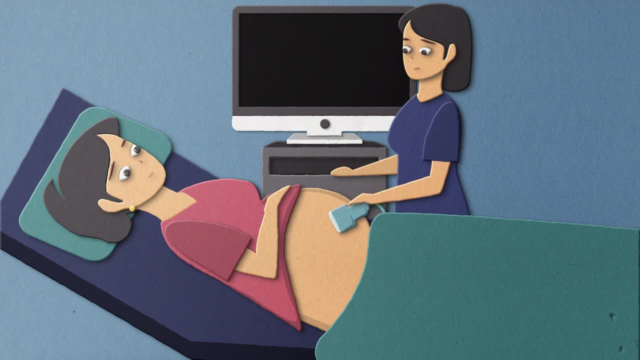 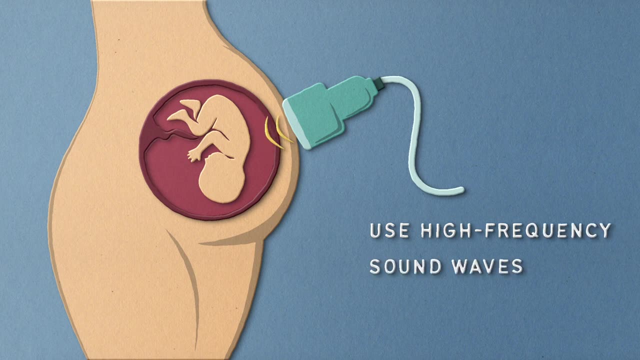 they have become more and more commonplace in the medical world, So if you have any questions, please feel free to ask them in the comments below. Ultrasound probes are a very useful tool in a wide range of diagnostic procedures. Ultrasound probes use high-frequency sound waves well above the threshold for human hearing. 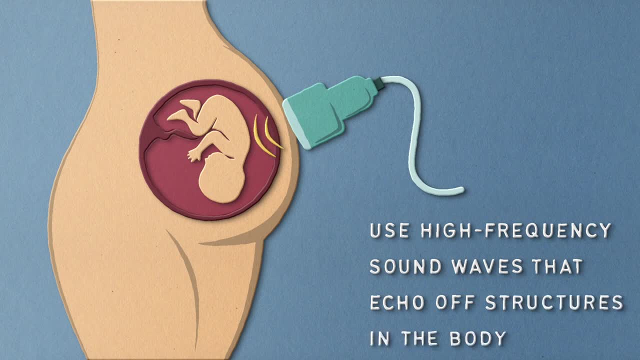 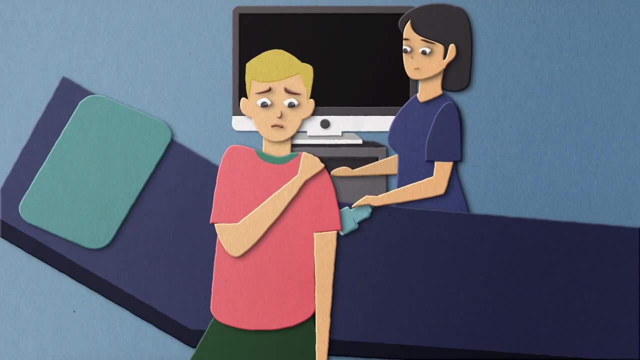 that echo off structures in the body. These reflected waves are then captured by a computer, creating an image. Ultrasounds can indeed be used for a range of imaging needs, For example in orthopedics to investigate problems. the ultrasound probe can be used to detect the 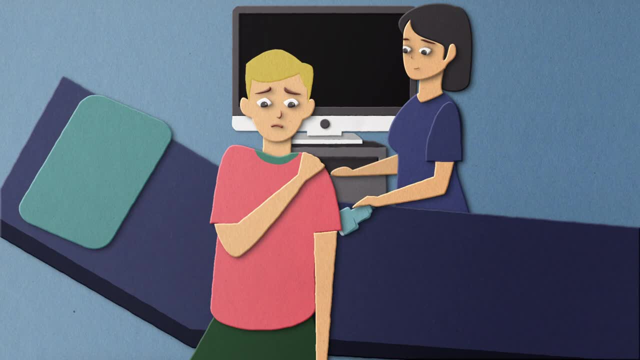 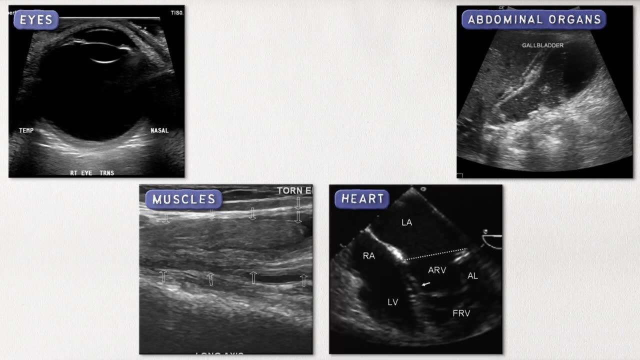 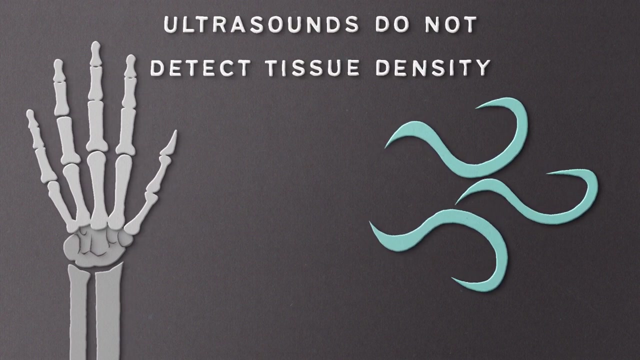 rotator cuff injuries. Doctors also commonly use ultrasounds to image the eyes, muscles, abdominal organs or heart. Ultrasounds do have their limitations, though, Since they do not detect tissue density structures that readily reflect echoes, but have very different densities. 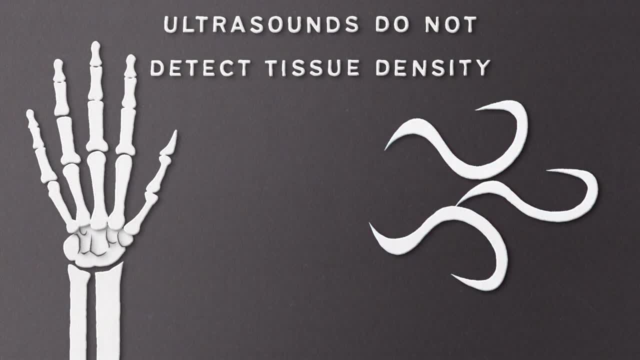 such as bone and hair may both appear white on the ultrasound. Last, but definitely not the last, but we are almost at the end of this video. If you have any questions, leave a comment below and we'll answer them in the next video. Until then, take care and take care.